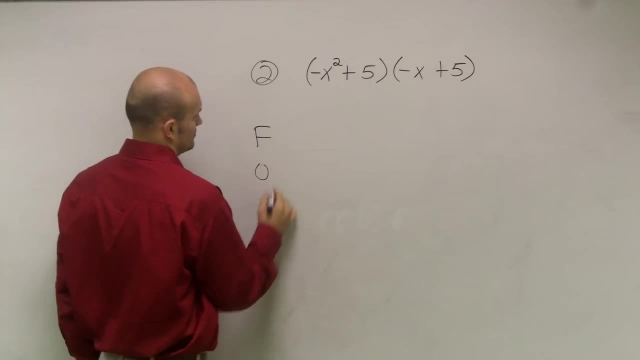 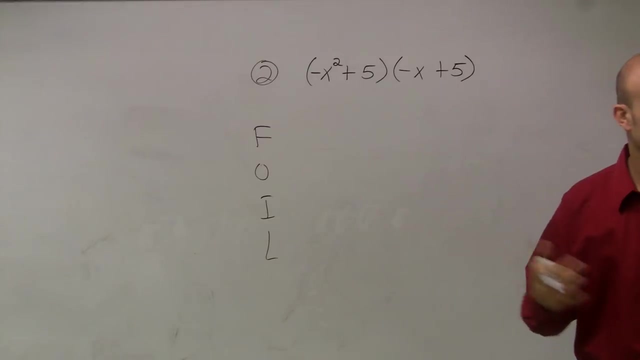 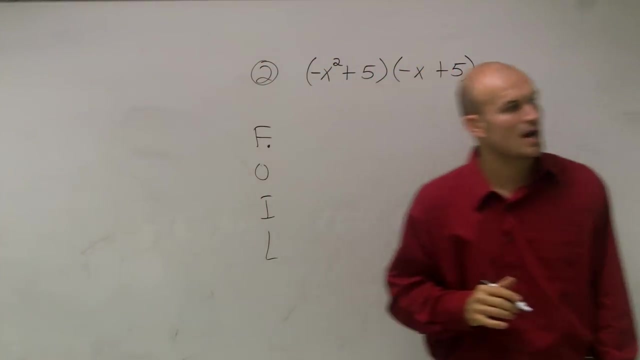 word And the special word we're going to memorize is FOIL, And hence this is also going to be called the FOIL technique. So why are we going to use FOIL and what does FOIL represent? FOIL represents our placement and how we're going to multiply our certain 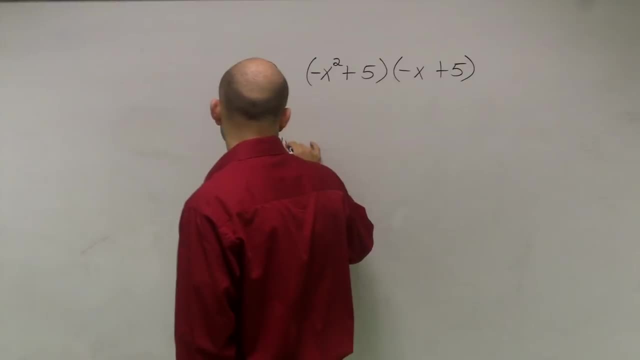 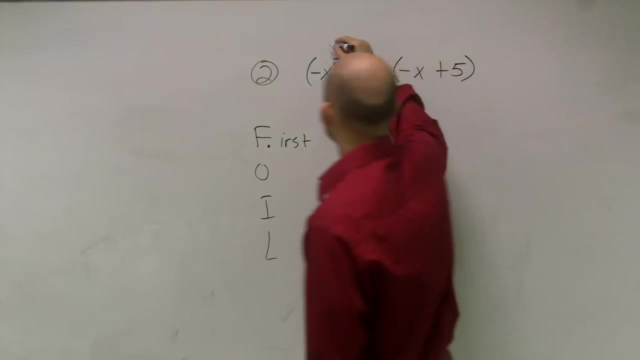 terms. So the first one, F, represents first. So what that means is I'm going to multiply the first two terms of each binomial. So what I'm going to do is I'm going to put a little F in front of or above my two first terms, so you guys can understand what are. 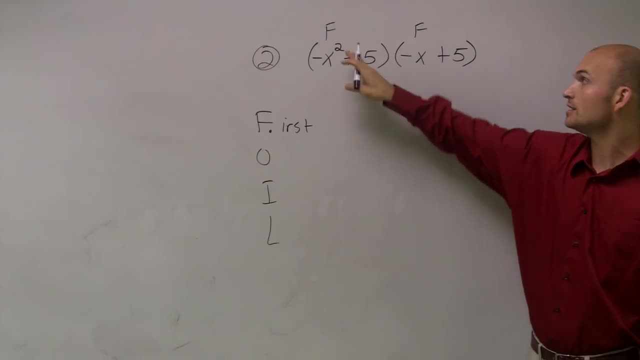 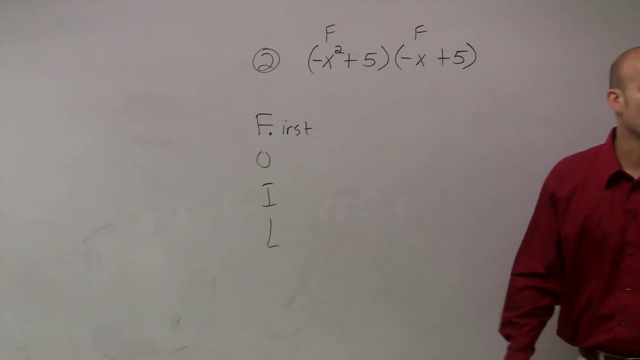 the first terms. If you look at the first binomial, If you were to read from left to right, you'd notice that negative x squared and negative x are the first terms in each binomial. Does that make sense? O represents outer, or I just like. 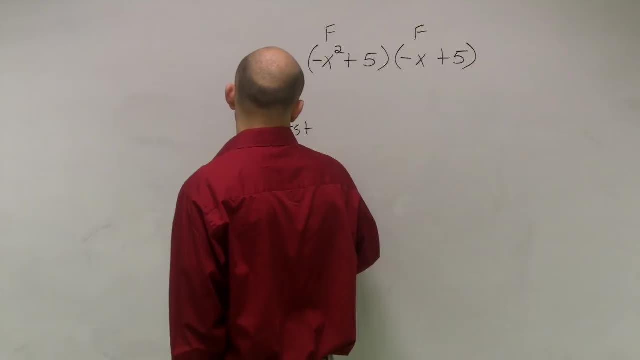 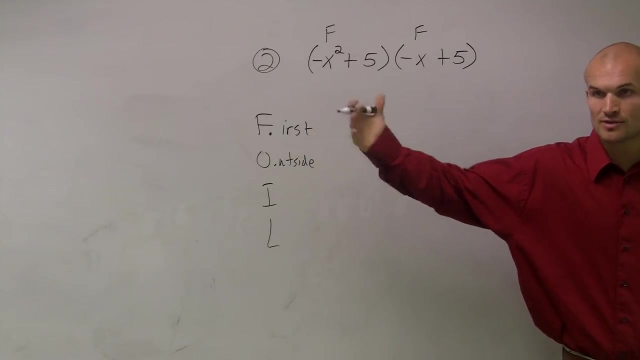 to call them outside terms. So if you look at your binomial, if you look at this expression as a whole, the farther outside terms or the farther outer terms are going to be x squared and 5.. Those are on the outer edges, right? 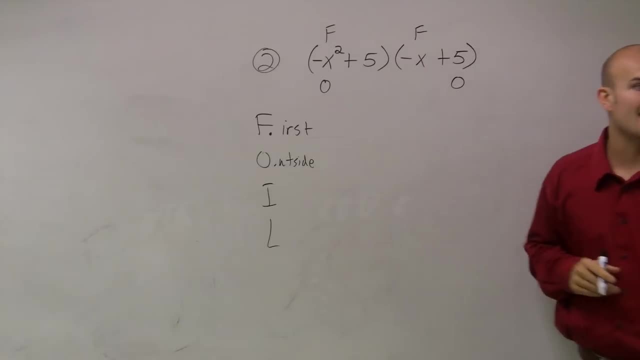 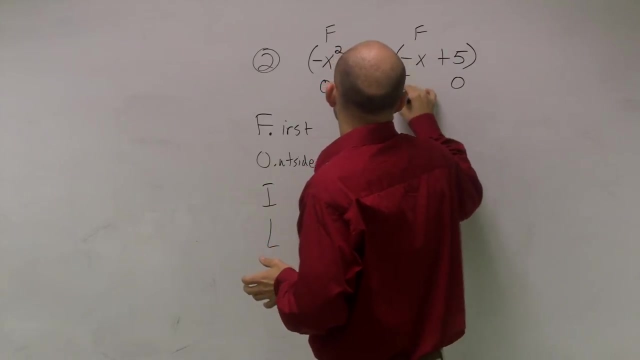 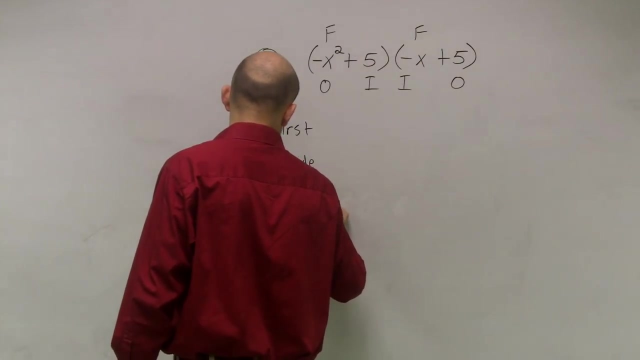 So that's why those are going to be called my outside terms. Then i represents the inside terms If those are on the outer, which 5 and negative x are going to be on the inside terms. So I just call these inner or the inside. 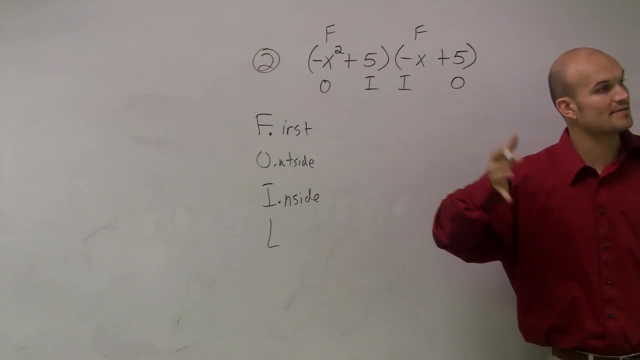 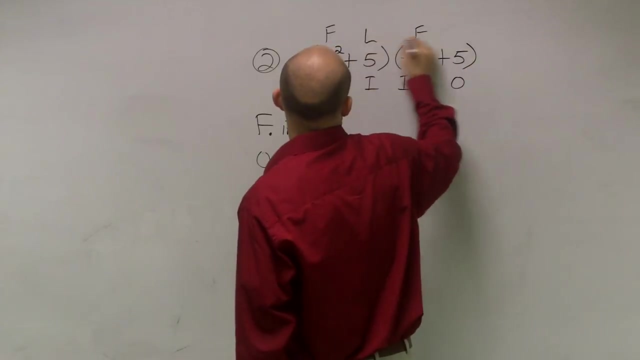 And then l represents the last. So again, if you're reading from left to right, if these two are your first two terms you read, these are going to be the last two terms you read. Now, ladies and gentlemen, all we're going to do. 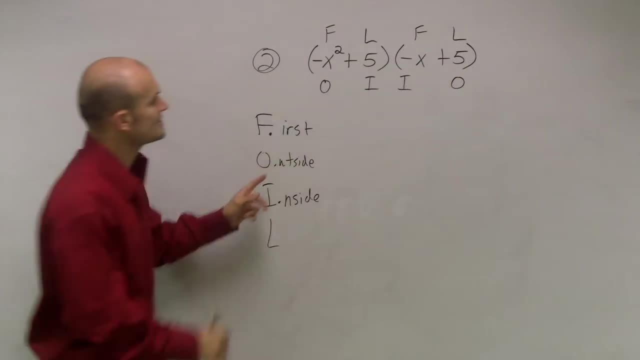 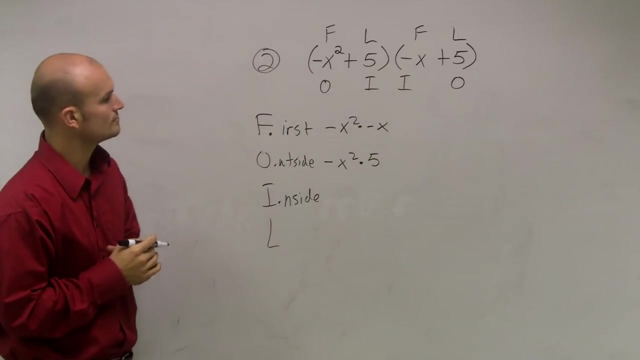 is just multiply each one of those terms. So the first I said to multiply negative x squared times negative x. So just write it out: negative x squared times negative x. Outside: multiply these terms: negative x squared times 5.. Inside: 5 times negative x. 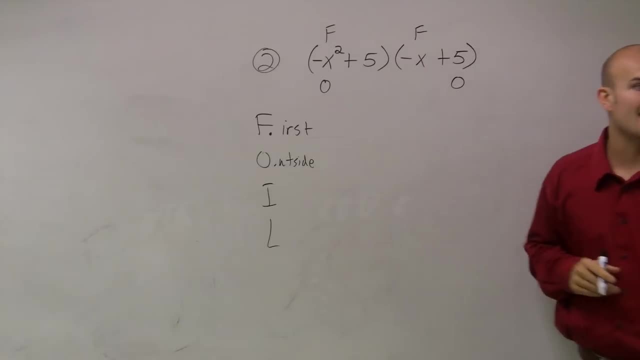 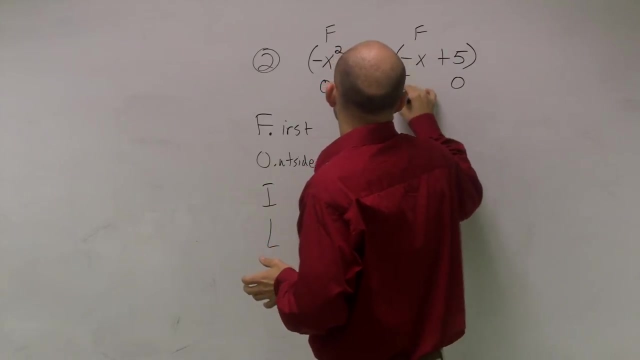 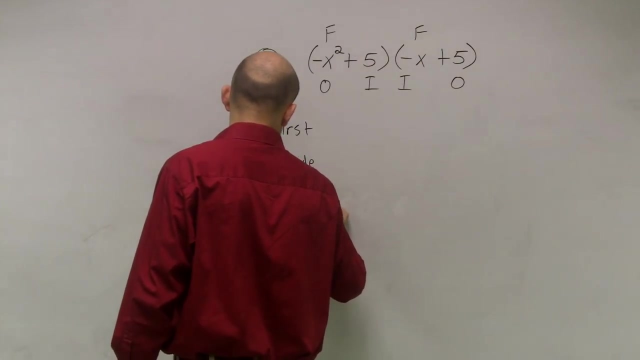 So that's why those are going to be called my outside terms. Then i represents the inside terms If those are on the outer, which 5 and negative x are going to be on the inside terms. So I just call these inner or the inside. 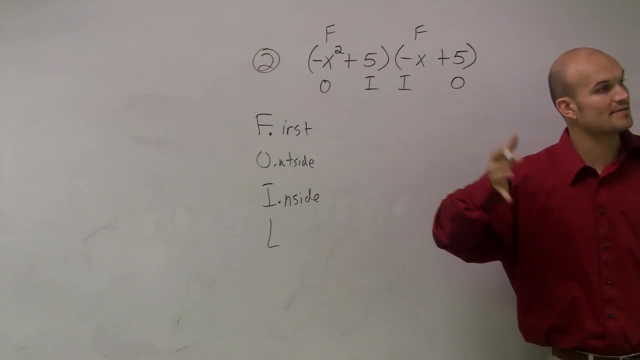 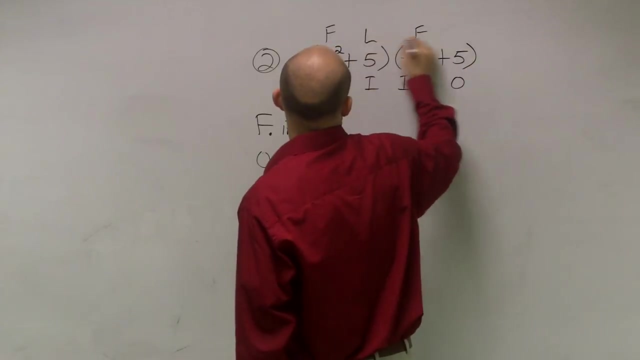 And then l represents the last. So again, if you're reading from left to right, if these two are your first two terms you read, these are going to be the last two terms you read. Now, ladies and gentlemen, all we're going to do. 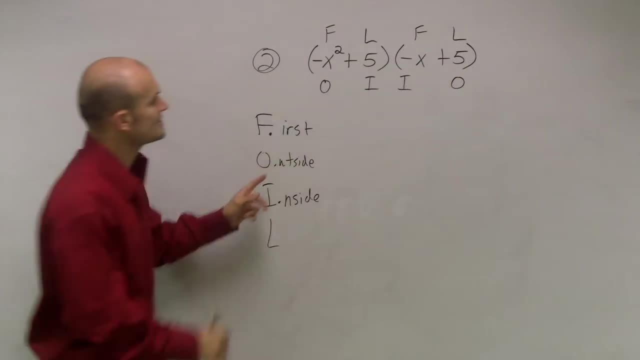 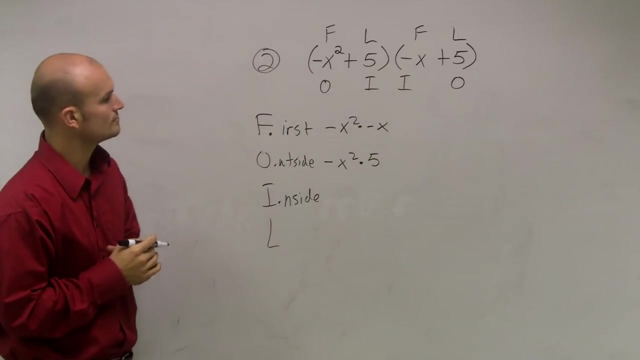 is just multiply each one of those terms. So the first I said to multiply negative x squared times negative x. So just write it out: negative x squared times negative x. Outside: multiply these terms: negative x squared times 5.. Inside: 5 times negative x. 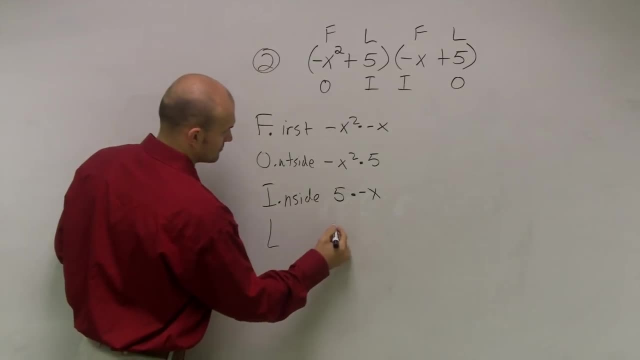 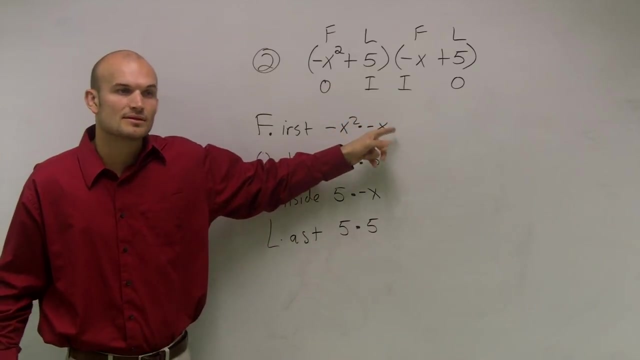 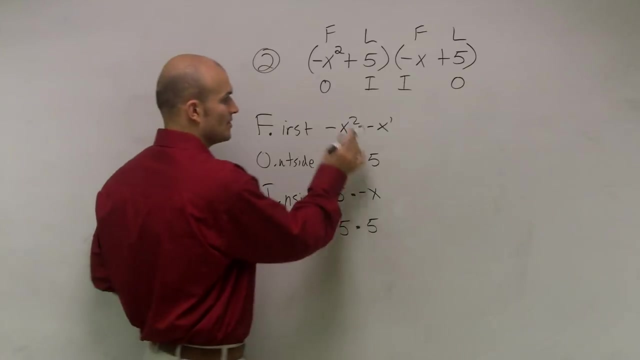 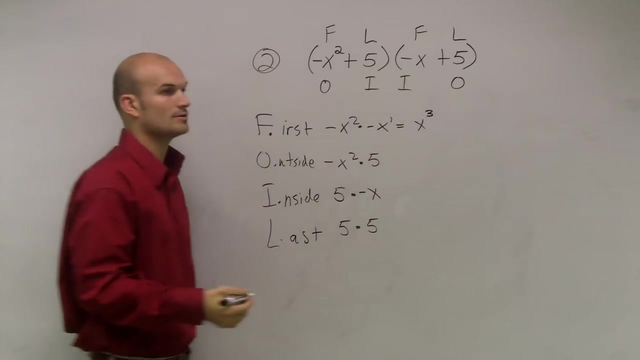 And last 5 times 5.. OK, negative x: squared times negative x. Remember there's an exponent here. We need to add the exponents right. Add the exponents A negative times a negative provides a positive. So you have x to the third power, right. 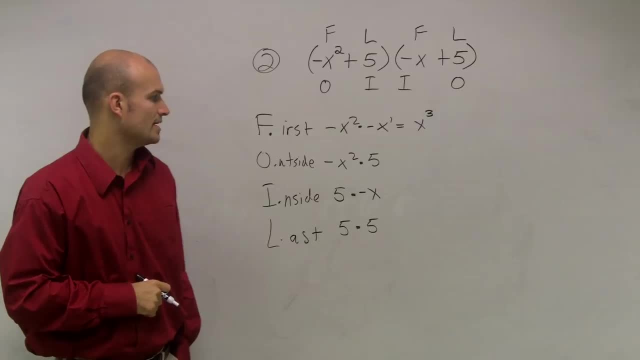 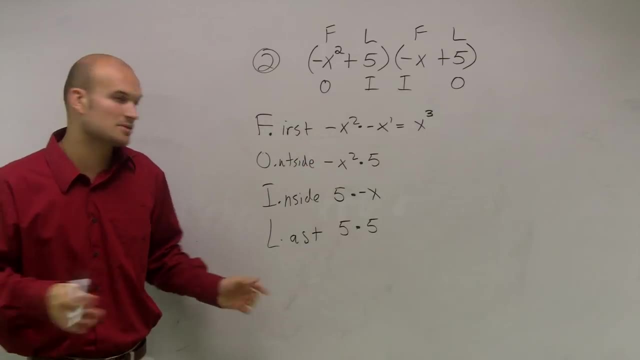 The negatives cancel out And I add my exponents because I'm multiplying them. Here. I'm multiplying a number, I'm multiplying a number times a variable. If you just multiply a number times a variable, it's just going to remain your number times a variable. 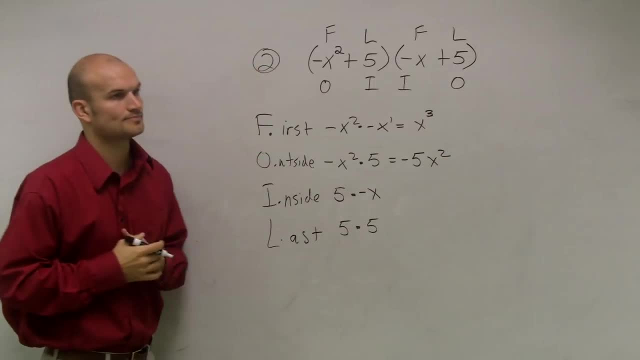 So this becomes now a negative 5 x squared. What was wrong? No, I was just wondering if you were right. I don't know. I don't have a writing apparatus. You did Whatever. I used to build my word. 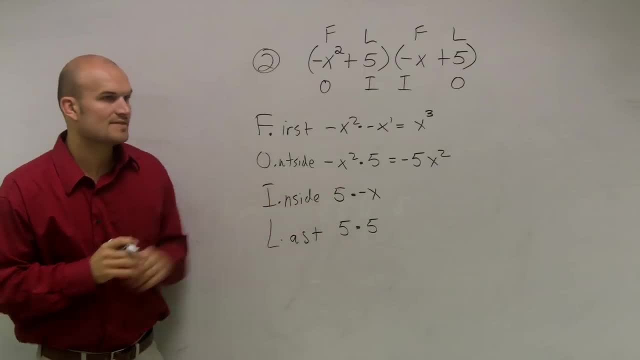 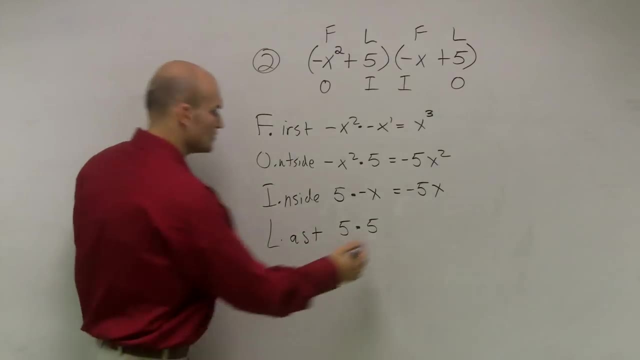 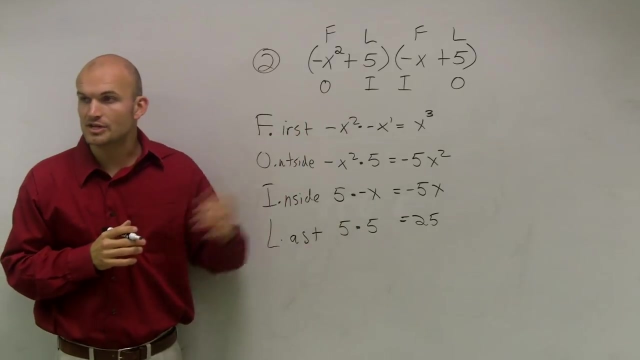 You got it together right. So here comes the inside. Inside: 5 times negative x is equal to a negative 5 times x, And then the last 5 times 5 equals 25,. all right, So now, ladies and gentlemen, all we simply need to do: